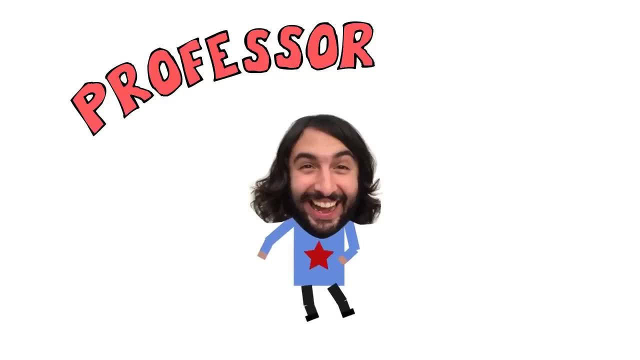 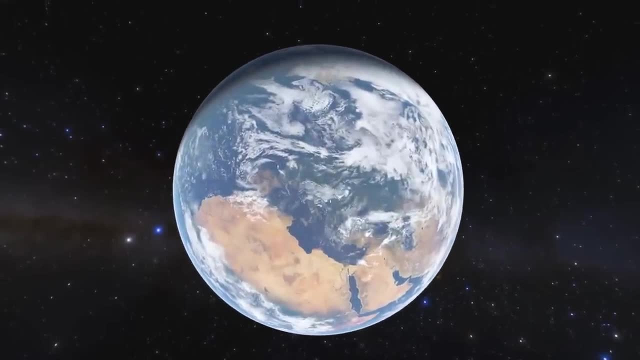 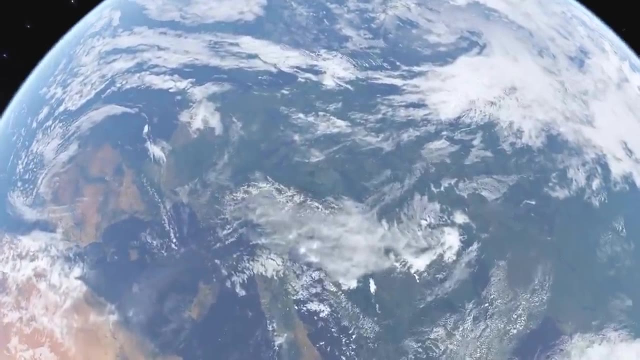 This is Earth, a rocky planet, covered with liquid water, orbiting within the habitable zone of a very typical star. From afar, it may not look like much, but if you get close enough, it becomes quite clear that there is a lot to study on this little blue world. 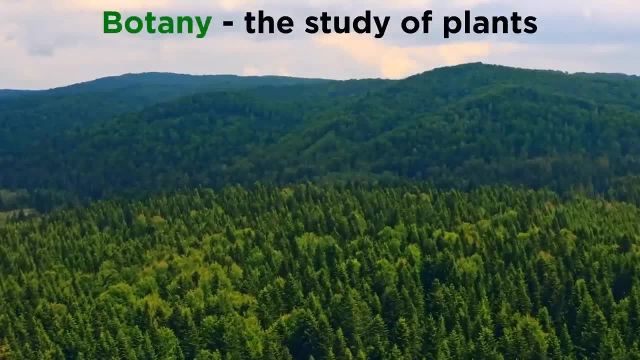 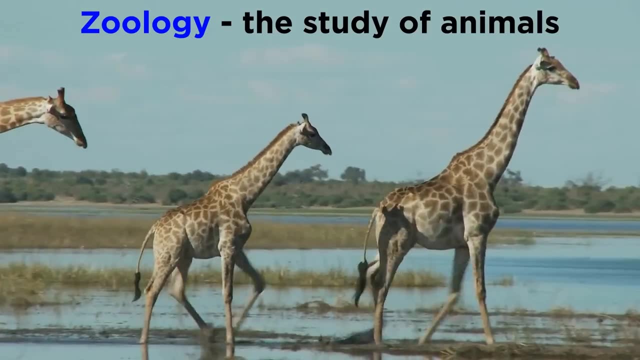 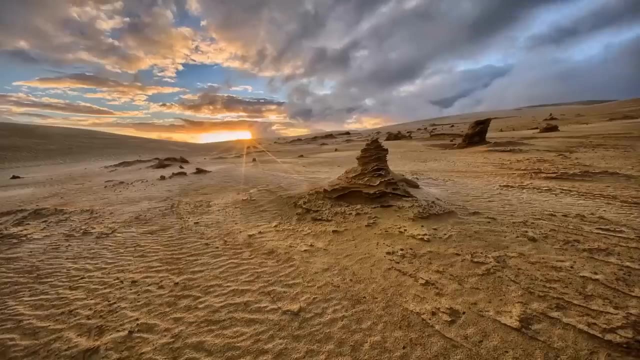 Some choose to study botany to learn about the wide variety of plant life. Some study zoology and learn about all the animals walking on the land, flying in the air, and swimming in the ocean. But some choose to study the Earth itself. What is the precise composition of the Earth? 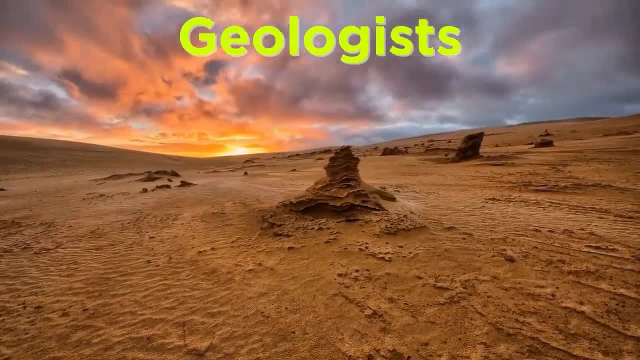 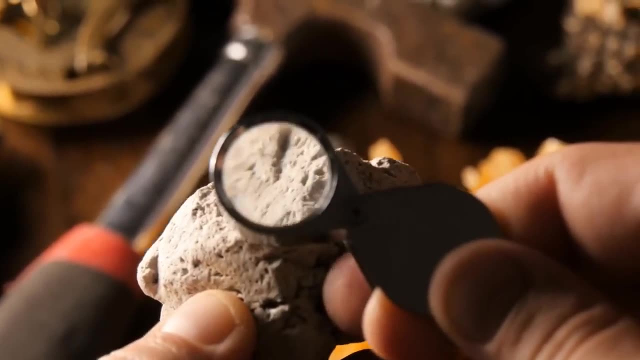 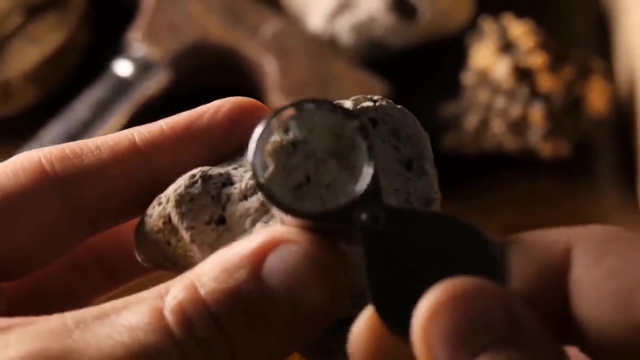 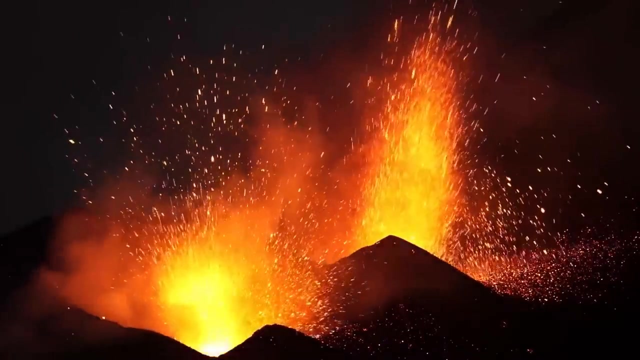 What is its history? The people who answer these questions are geologists. Now, when most people think of a geologist, they tend to imagine someone examining a bunch of rocks. And of course, geologists do indeed study rocks. But geology is also much more than this. To understand why earthquakes occur or how volcanoes form, one must do more than simply look at rocks. 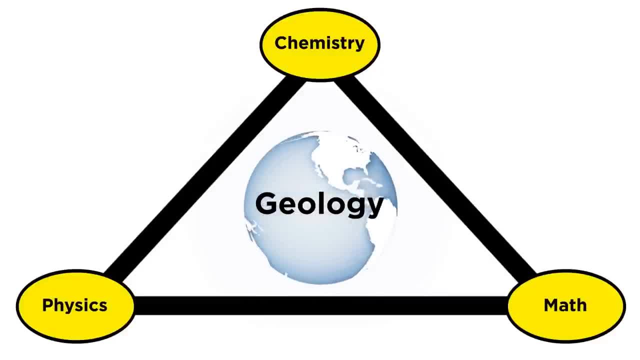 At its core, geology is a multidisciplinary science that combines chemistry, physics, and mathematics to investigate an enormous variety of processes that occur on and in the Earth. As we will come to understand in this series, 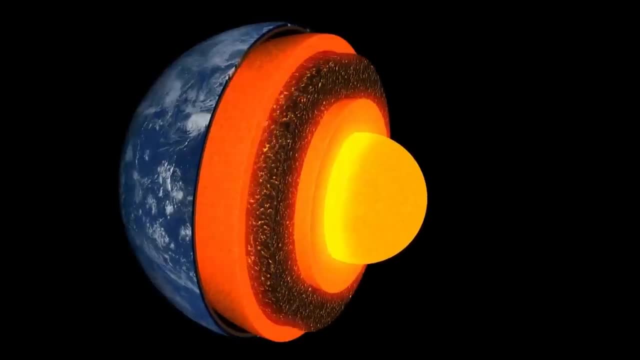 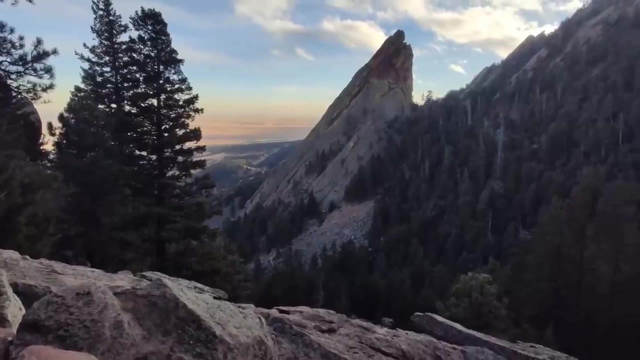 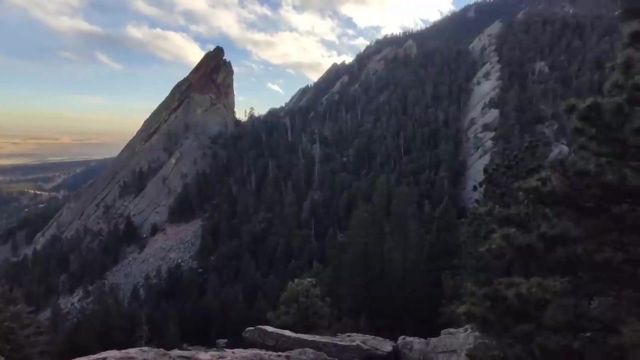 geology encompasses every aspect of Earth's structure, from the molten iron core to the beautiful minerals we find on its surface. Much of what geologists study transpired over incredibly long timescales, originating anywhere from thousands to billions of years in the past. 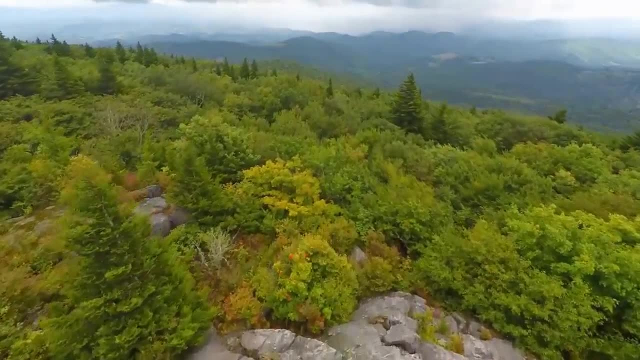 Geologic processes have shaped the entire world, and geologists have been doing so for a long time. For example, the Appalachian Mountains of eastern North America contain limestones, 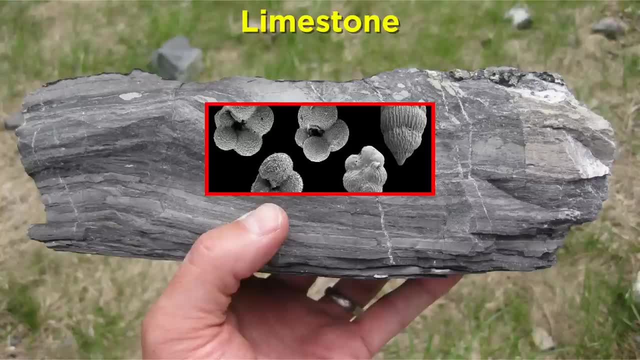 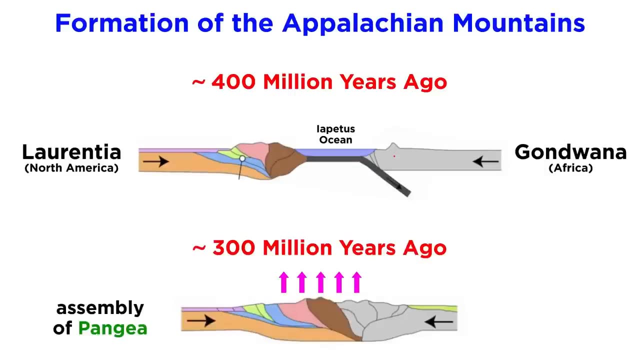 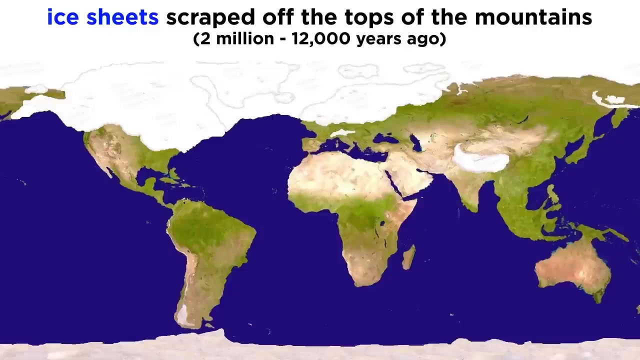 which are composed of the shells of marine animals that lived there, in a shallow ocean more than 400 million years ago. Then, 300 million years ago, those rock beds were thrust upwards as Earth's tectonic plates began to converge along the eastern U.S. coast. Later, during glacial periods between 2 million and 12,000 years ago, the earth's tectonic plates began to converge along the eastern U.S. coast. Later, during glacial periods between 2 million and 12,000 years ago, mile-thick ice sheets scraped off the tops of these mountains, like huge bulldozers, as they moved 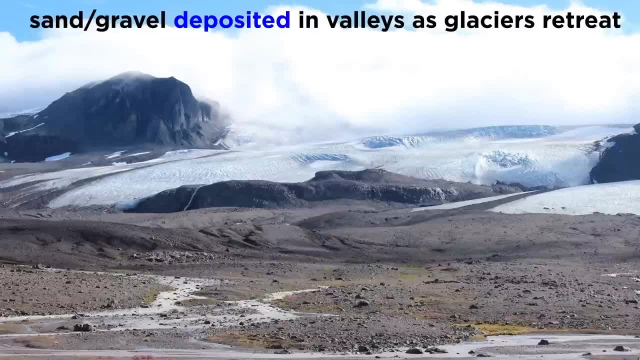 southward, then deposited hundreds of feet of sand and gravel in stream valleys as they retreated 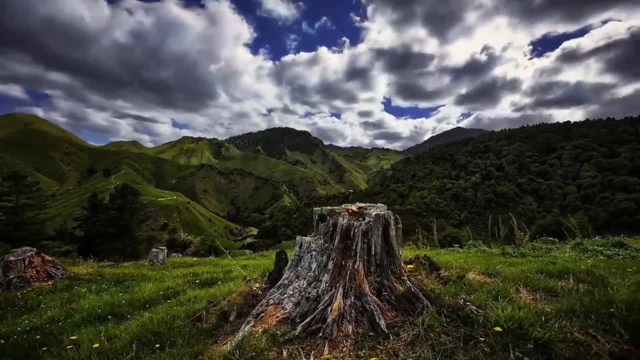 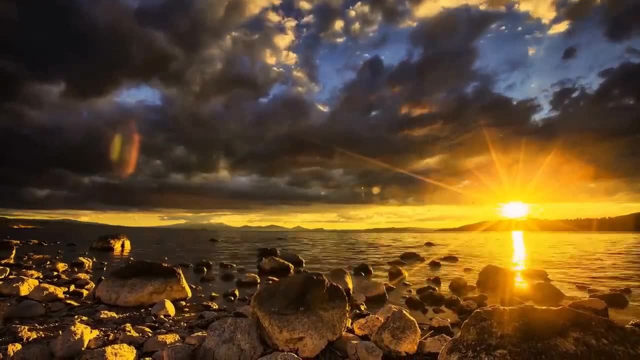 northward and melted. How is it that we can know these things, exactly? And furthermore, why even bother studying geology if all these phenomena occur on a much longer timescale than humans can observe during their lifetimes? 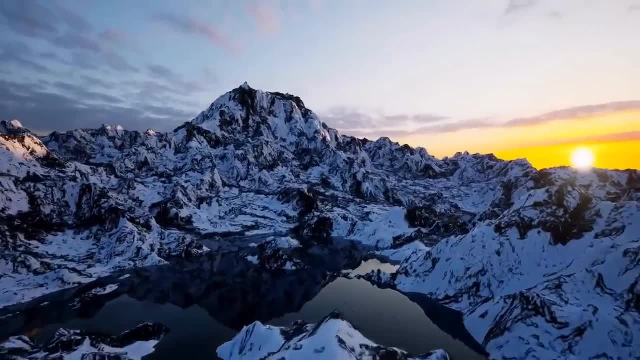 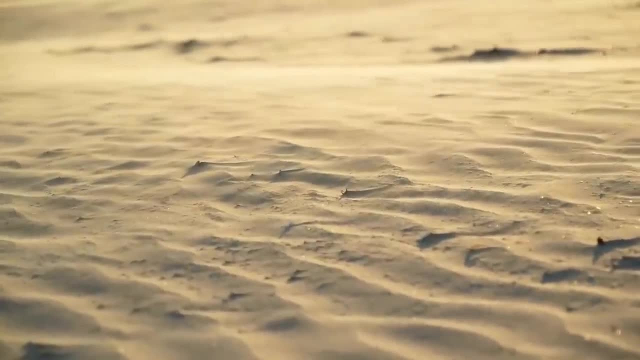 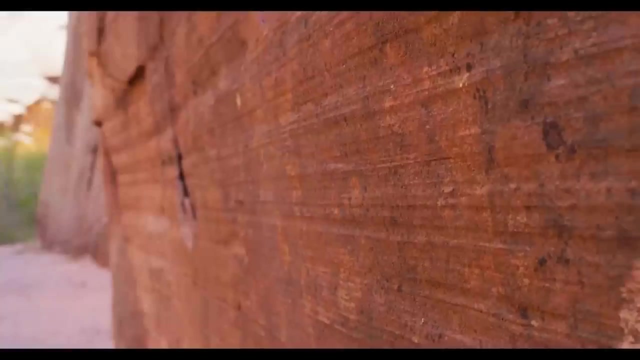 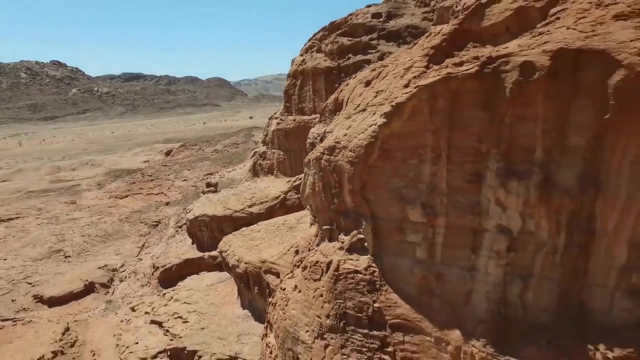 The answer is that the processes that shaped our planet billions of years ago still occur today and can be easily observed and measured. Next time you visit the beach, pay close attention to the patterns of the sand and observe them as they form from wind and water currents. These patterns are exactly what we find in many ancient sandstones, therefore it is reasonable to assume they were created by the same processes, just at different points in time. This is the essence of the 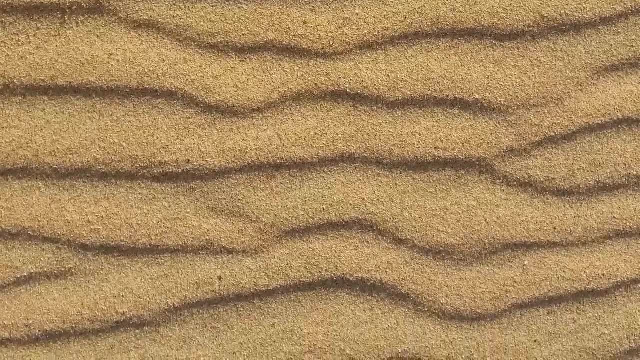 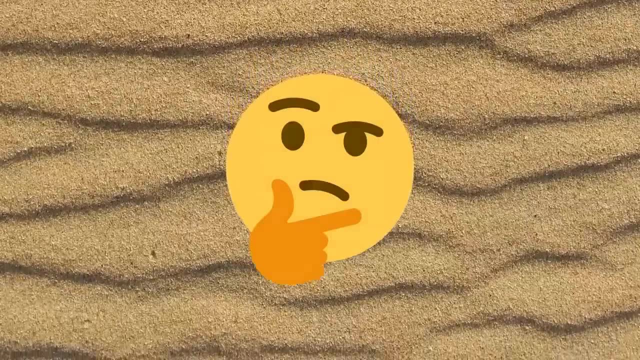 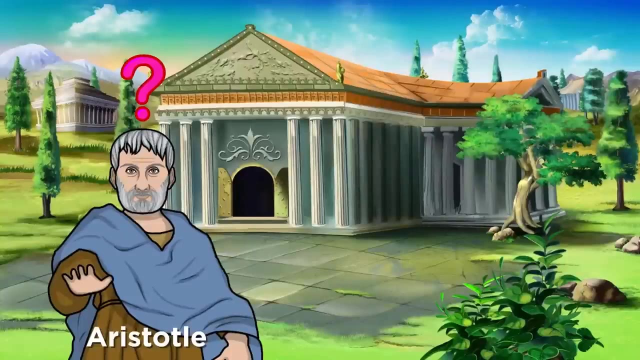 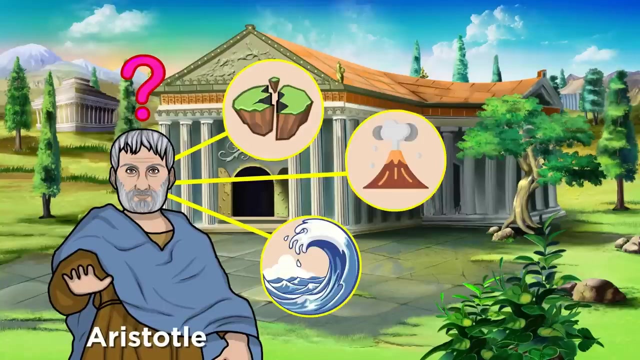 geology. Observing beach sand form ripples and dunes may not be the most exciting activity to most, so you might be wondering who would be interested in geology. The first recorded dabbling in geology was by Aristotle and the ancient Greeks. These ancient philosophers wanted to understand natural phenomena, especially those impactful to human life, like earthquakes, volcanoes, and tidal waves. Aristotle thought earthquakes were caused by 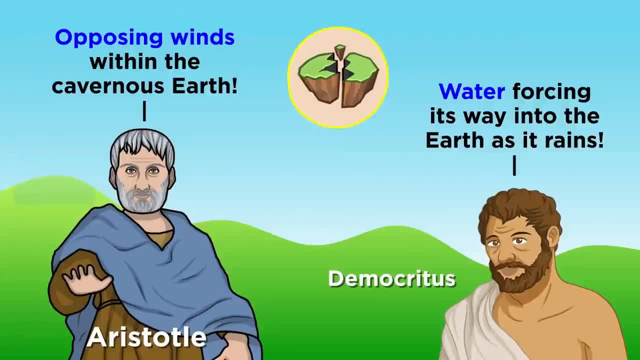 opposing winds, and he thought that earthquakes were caused by opposing winds, and he thought that the cause was water forcing its way into the earth as it rains. Obviously, these are both 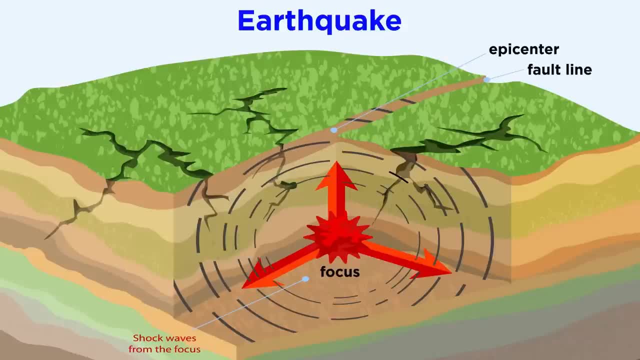 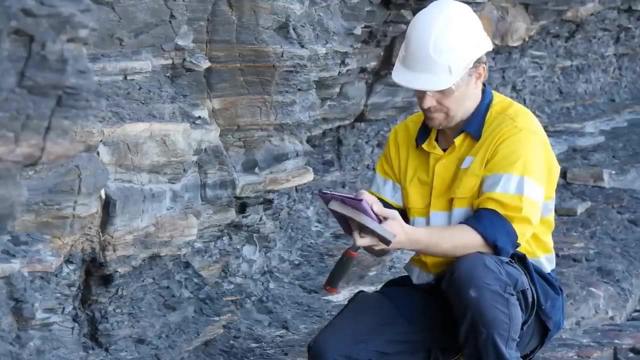 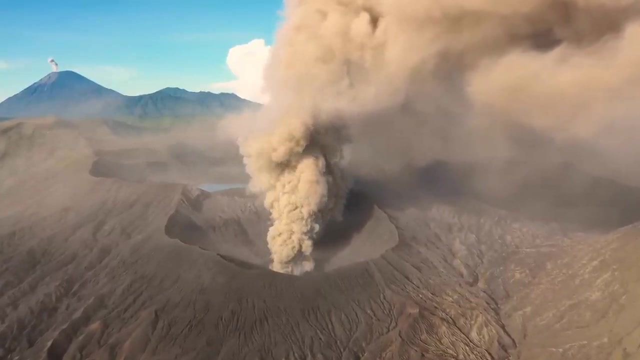 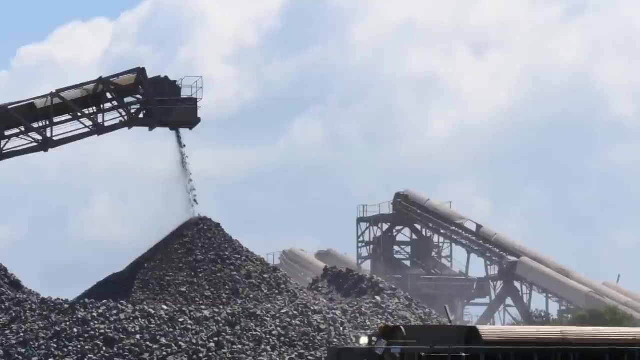 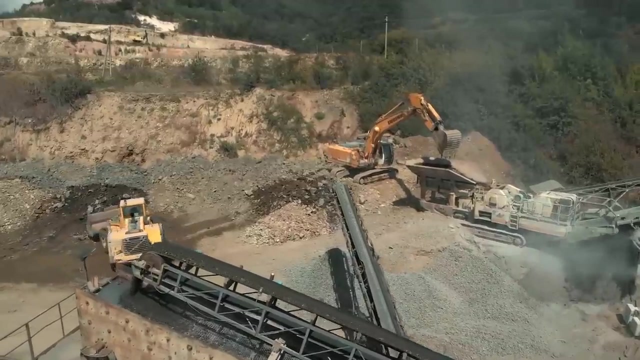 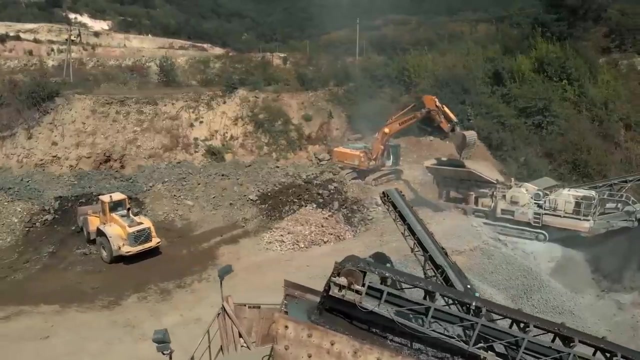 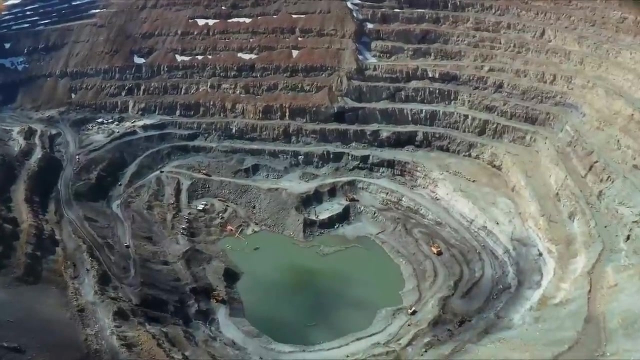 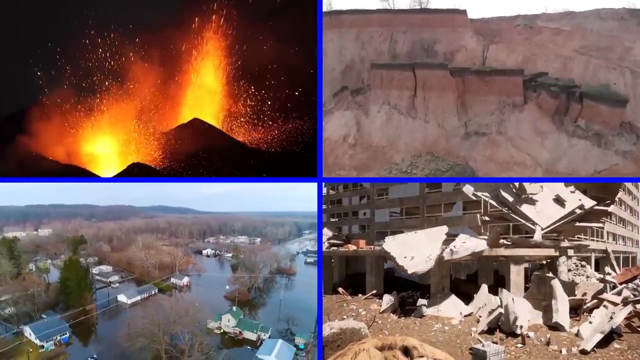 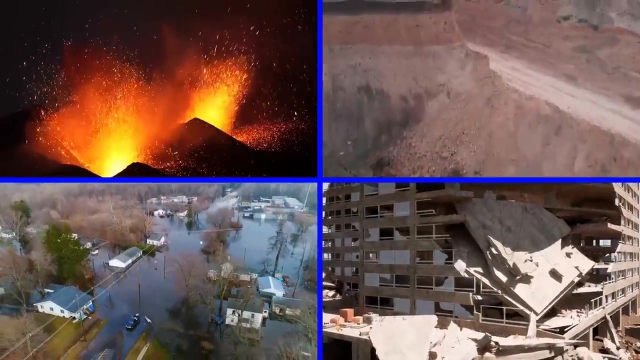 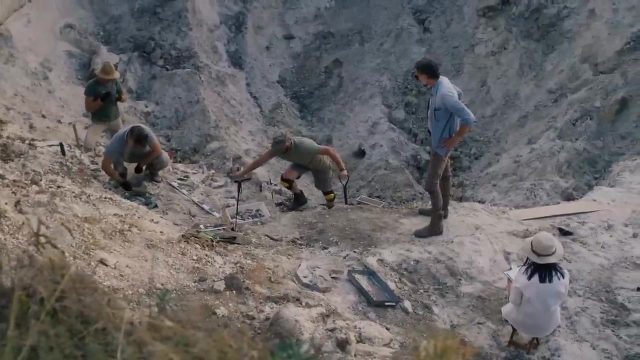 incorrect, and we now know earthquakes to be caused by rocks cracking under the enormous stress created by plate tectonics, but the desire to understand is ancient. Geology has come a long way since the time of Aristotle and has many applications toward improving and protecting human life. For example, volcanology has been a great source of information for us to understand, geologists, or geologists who study volcanoes, closely monitor active ones and create early warning systems to evacuate towns before any volcanic eruptions. Furthermore, earth contains minerals, metals, and sources of energy that we have used to build and power the technology and infrastructure responsible for raising our collective standard of living over the past few hundred years. In fact, many geologists work in the resource industry, finding new places or developing new ways to extract minerals and energy. Others assess hazards to human life, like the volcanic eruptions we mentioned, but also slope failures, massive floods, and structural damage from earthquakes. Biologists interested in the evolution of life on earth work closely with geologists in looking at the rock record to find the fossils and footprints of organisms that are now long extinct. 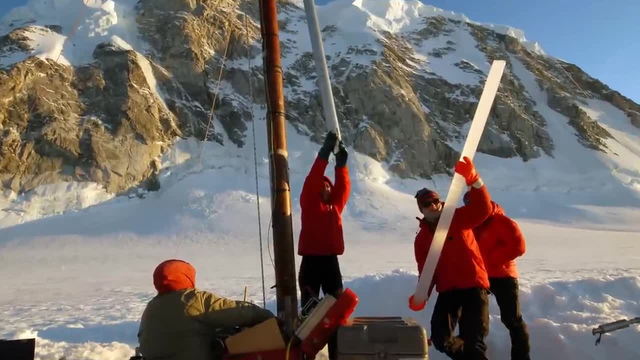 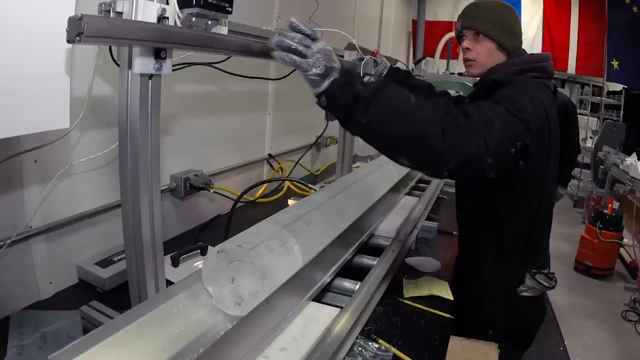 Climate scientists interested in understanding our impact on the environment measure, among other things, greenhouse gases trapped inside tiny bubbles from 800,000-year-old ice cores. 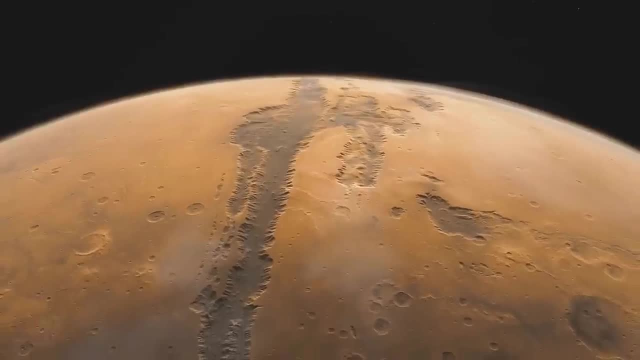 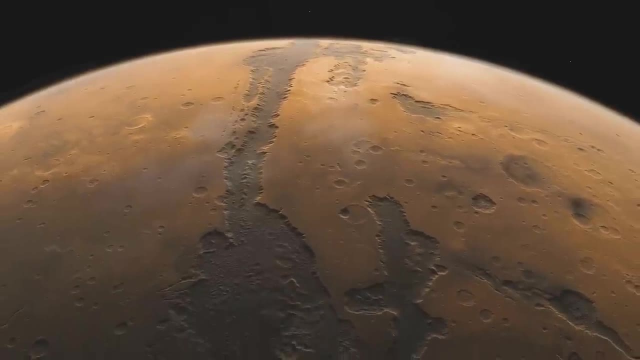 The impact doesn't even stop at our own planet. The understanding of earth provided by geologists acts as the framework that planetary scientists use to study outflow channels on Mars, crater потом sun, crater topography on the moon, Frage-Qui brandarowicz's paper about brain-dead englad... de も bage 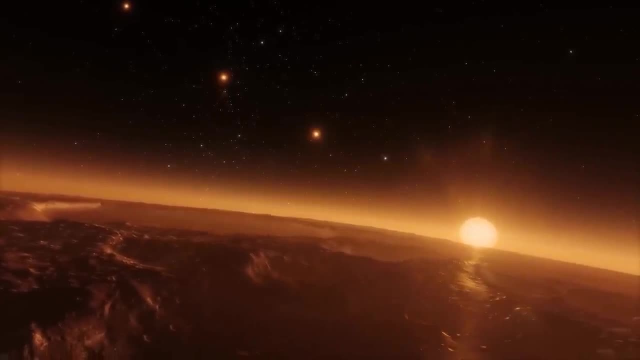 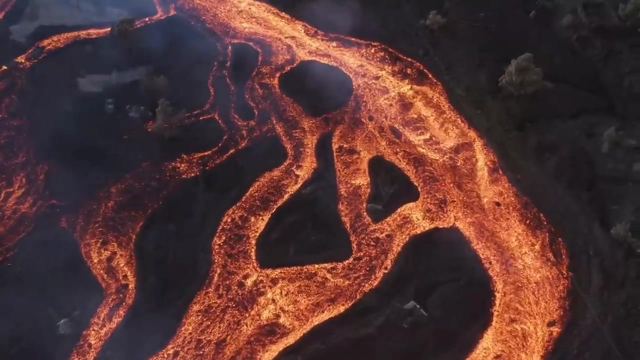 features of exoplanets that are continually being discovered. So as you can see, geology is not just about looking at rocks. It is as rich and multifaceted as any other scientific discipline. 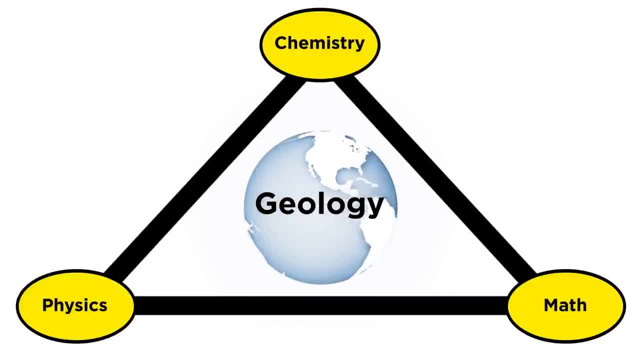 As we mentioned, geology utilizes concepts in chemistry, physics, and mathematics, and an